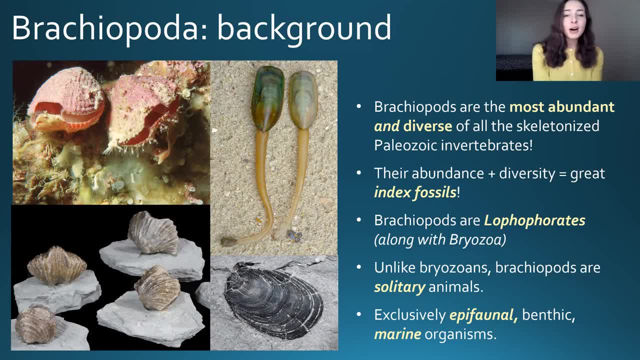 fossils during this era, as well as other times throughout Earth's history, and brachiopods are part of the group Lophophorates, along with bryozoans, which we went over in the last video. Unlike bryozoans, however, brachiopods are solitary animals rather than colonial. 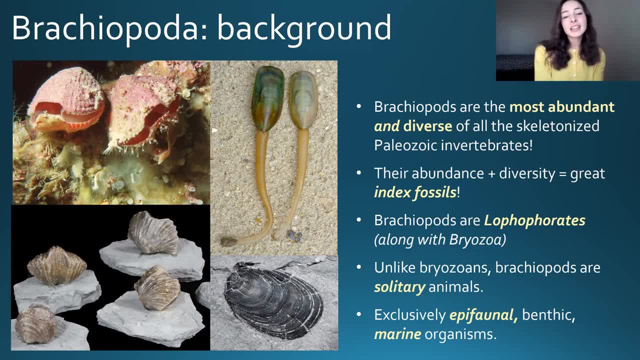 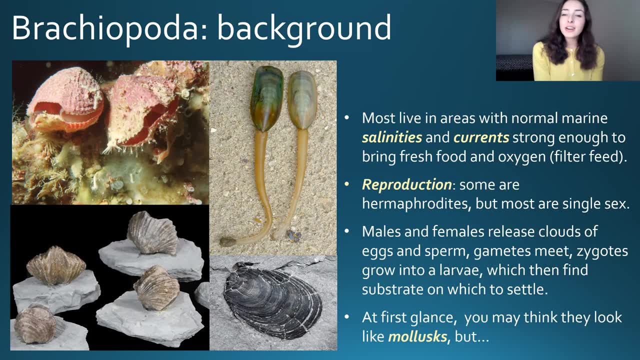 and they're exclusively marine and epiphanal, meaning that they live on the bottom of the ocean floor on a substrate. They have to be attached to a substrate. Most live in areas of normal marine salinities and with currents strong enough to bring fresh food and oxygen. 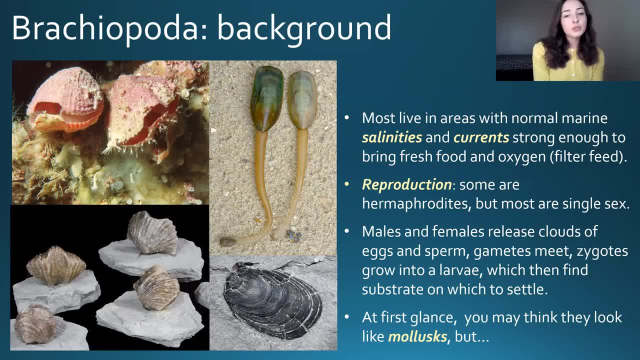 to filter, feed and to excrete their waste. And in terms of reproduction, some brachiopods are hermaphrodites, or both female and male, but most are male or female, and males and females release clouds of water. So they're very, very strong and they're very, very strong and they're very 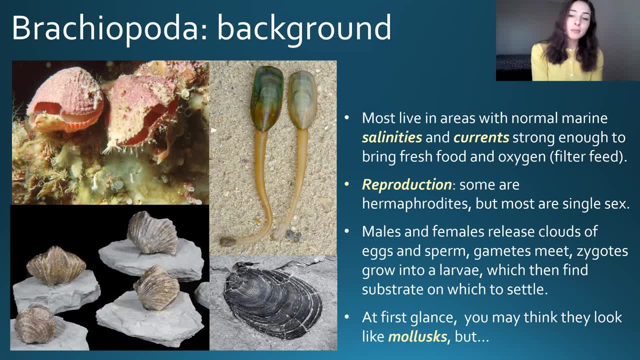 of eggs and sperm to reproduce, in which these eggs and sperm meet and form zygotes which grow into larvae, which then find a hard substrate to settle down on. And in terms of how these brachiopods look, we can see here on the top left an image of some articulate brachiopods in life. 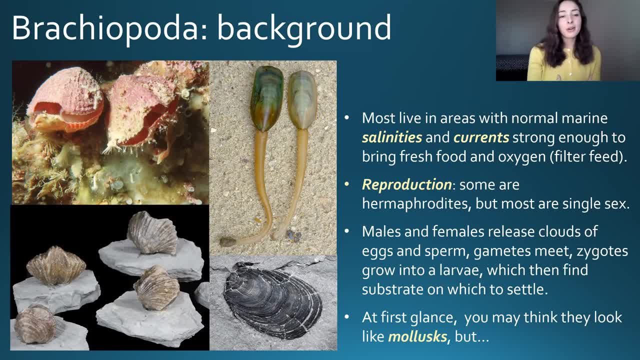 and we'll talk about the difference between articulate and inarticulate brachiopods, which we see on the top right side of this picture later in the classification section, And then at the bottom we see two pictures of fossilized articulates and inarticulates respectively. 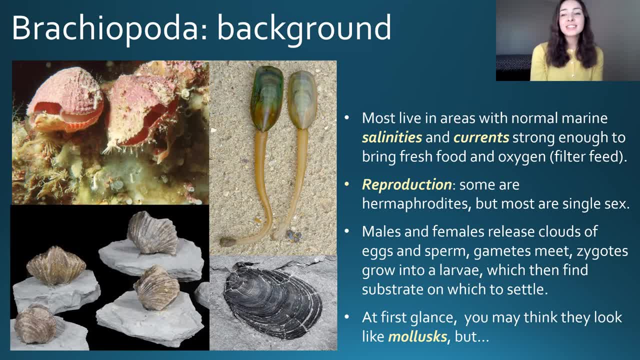 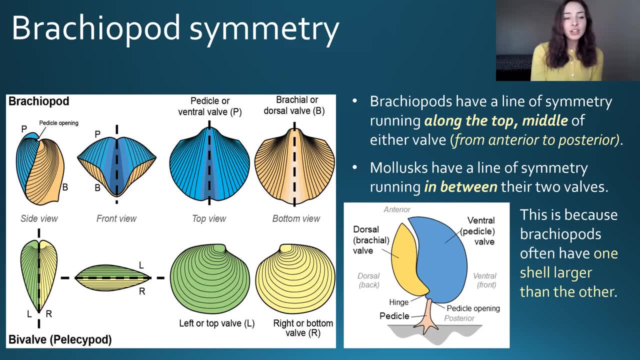 And at first glance you might think that these look like mollusks. but there's an easy way to tell the difference between brachiopod shells and mollusk shells. So on this slide we see on the left figure that brachiopods and mollusks have different symmetry. Symmetry is the easiest. 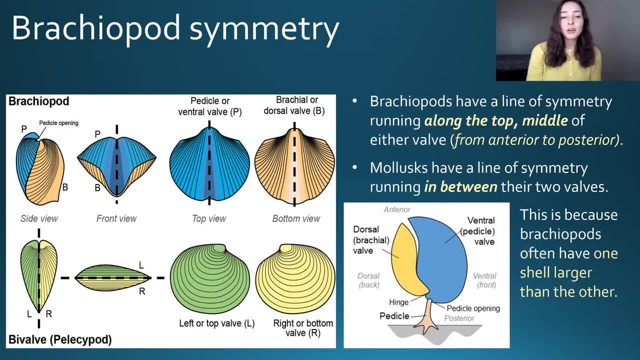 way to tell the difference between brachiopods and mollusks. What we can see is that brachiopods have a line of symmetry going along the top middle of their shell, whereas mollusks have a line of symmetry running in between their two valves of their shell. This is because, as we see, 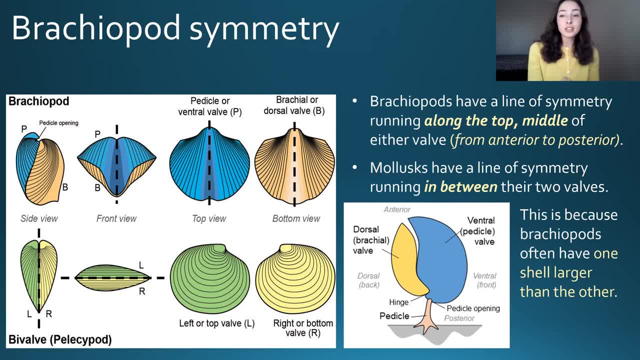 mollusks typically curve toward their hinge, and so they're not symmetrical along the top of their two shells. However, they are in between their two shells, whereas brachiopods are not symmetrical in between their two shells because they typically have one valve larger than the other. Now we can. 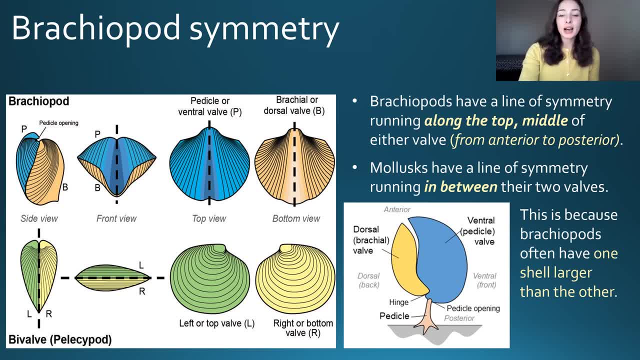 see an example of this when we look at the picture to the bottom right. What we have in this picture is a little cartoon of a brachiopod in life, where it's pedicle, which is what attaches it to its substrate, is attaching it, and then its shell has two valves. 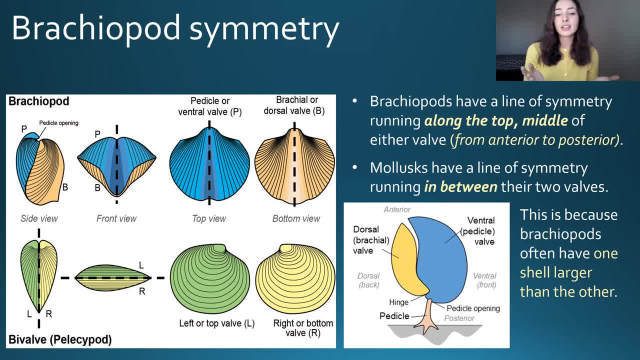 that open and close to feed on things. But these two valves are different sizes, As we can see. there's a ventral valve, or pedicle valve, which is in blue here, and this is the larger valve of the two, And then there's the dorsal or brachial valve, which is in yellow here. 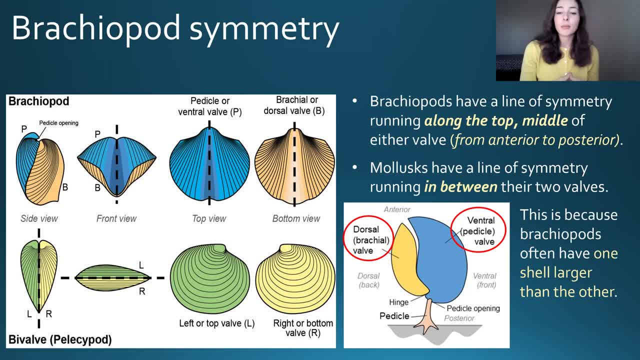 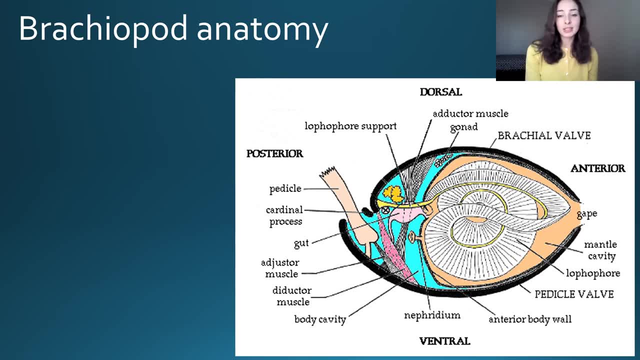 and much smaller than the ventral valve, which is a typical situation for brachiopods. So, getting into brachiopod anatomy, we need to talk a little bit about all these terms here. It looks really busy, but we're going to break it down step by step. First we have the brachial valve, or dorsal. 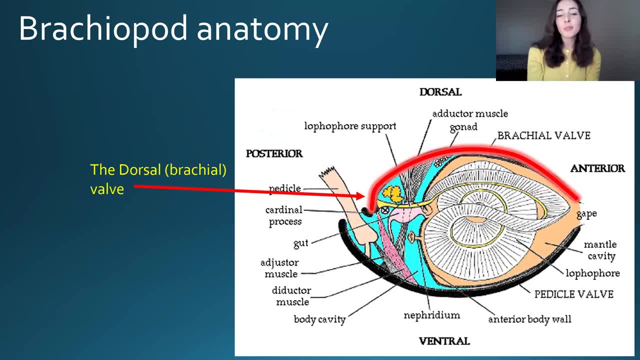 valve on top, outlined here in red, And this valve is called brachial because, as we'll see later, it is what the lofophore support attaches to, And we'll talk about the lofophore later, but, as we already know from the bryozoa video, the presence of a lofophore is why bryozoans and 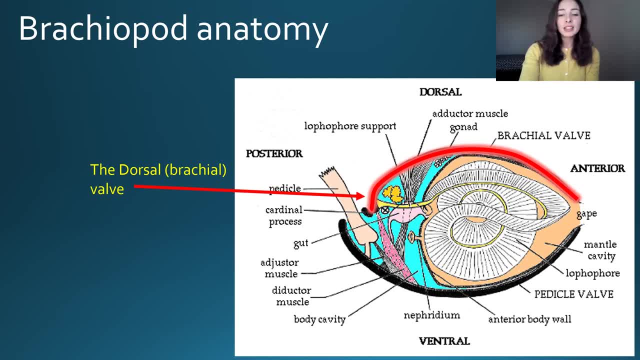 brachiopods are classified as lofophoreates, But before we get to that, we have the ventral or pedicle, which is called the pedicle valve, because the pedicle, which is that fleshy stalk that attaches the brachiopod to its substrate, that pedicle comes out of the pedicle valve or ventral valve. 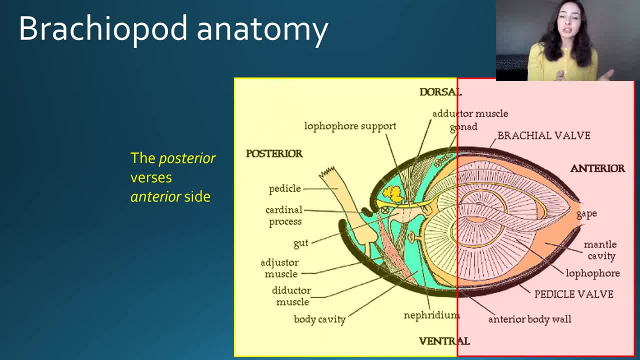 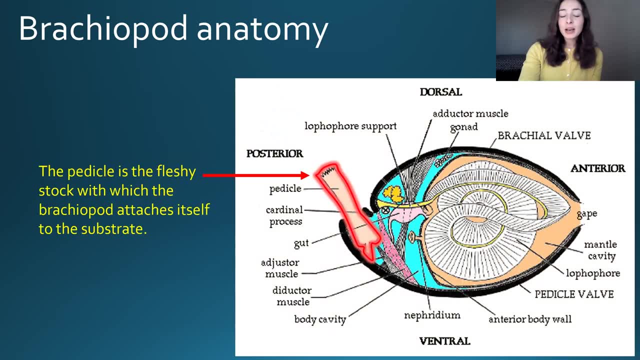 as we can see in this picture. And then we have these labels of posterior and anterior, which I just want to point out so that you're oriented the rest of the time we're labeling these features. Then we have the pedicle which I just mentioned, is the fleshy stalk which attaches. 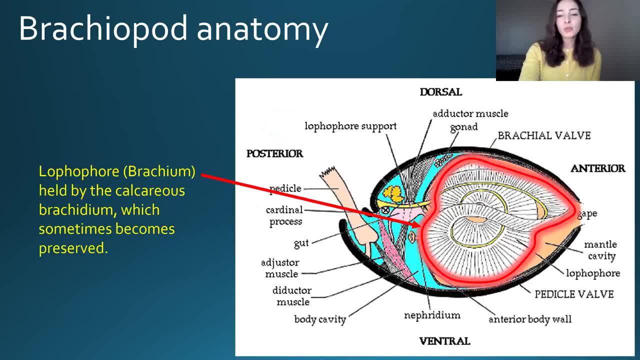 the brachiopod to its substrate. Additionally, we have the lofophore, which I also mentioned was a very distinctive feature of brachiopods and bryozoans and which is why they're classified as lofophoreates. Additionally, the lofophore is also sometimes called the brachium, which is why. 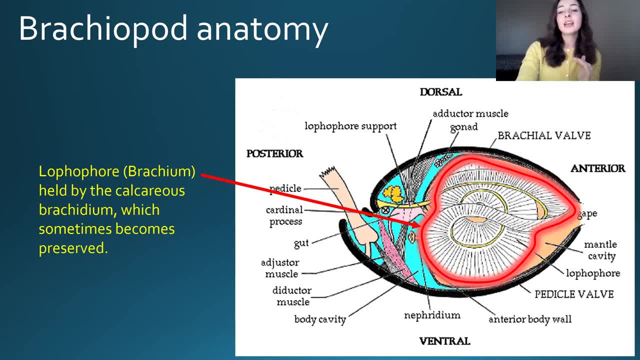 the brachial valve got its name because the lofophore, or brachium, is attached to that valve. Additionally, this lofophore is held in place by a lofophore support, which is pointed out here in yellow and highlighted now in this picture, And this support is calcareous and sometimes gets. 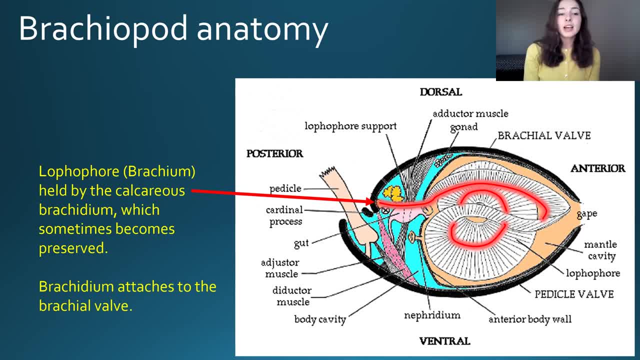 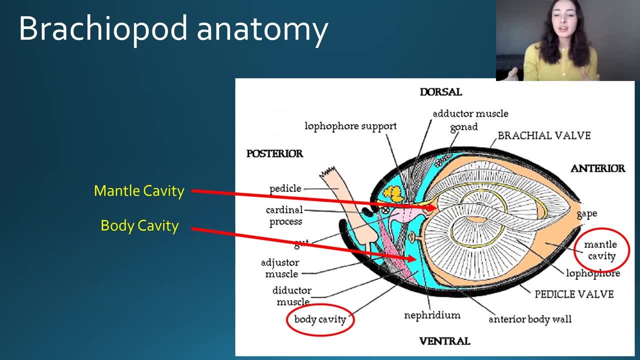 preserved, which later we'll see is sometimes used as a distinguishing feature when identifying brachiopods as fossils. Then we just have the difference between the mantle cavity in orange here, which hosts mainly the lofophore, and then we have the body cavity in blue, and this hosts 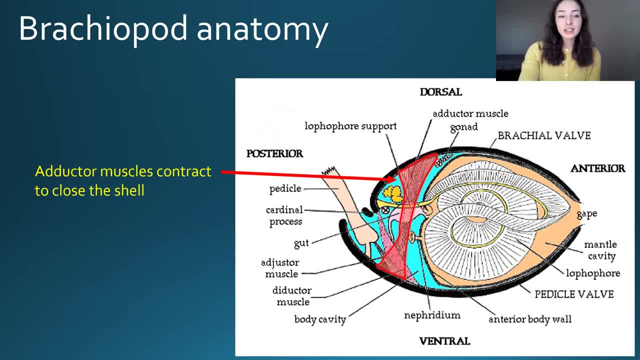 pretty much everything else in the animal, such as the adductor muscles which contract to close the shell, contrasting them with diaductor muscles which contract to open the shell. And because brachiopods have diaductors rather than just adductors like mollusks do, they don't automatically. 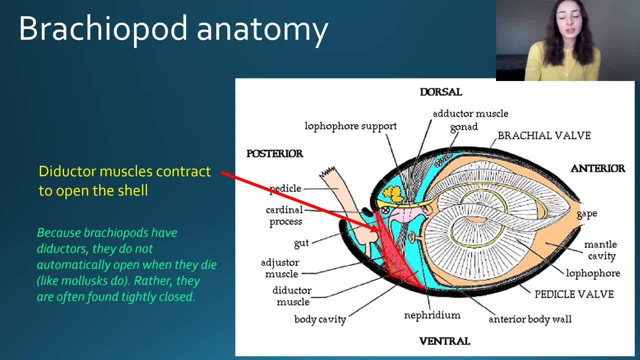 open when they die. Rather, they are often found tightly closed, which is actually another really easy way to tell between brachiopods and mollusks. in the fossil record, Brachiopods are typically found with both their valves, and mollusks are typically found with either one valve. 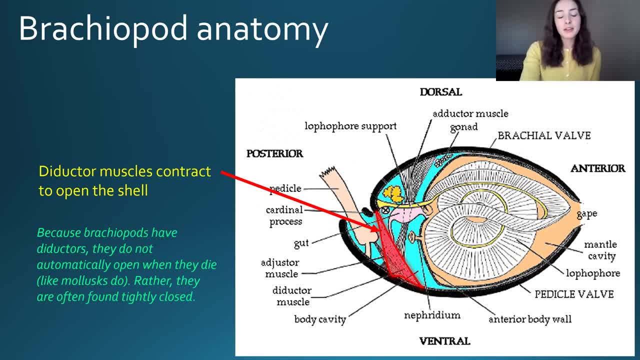 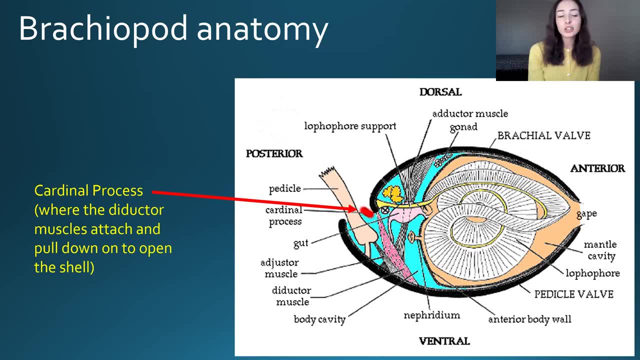 or just a fragment of a valve, and pretty much never with both their valves. Then we have what's called the cardinal process, which is a little part of the brachial valve which the diaductor muscles attach to in order to pull down on it and open the shell. Then we have adjuster muscles. 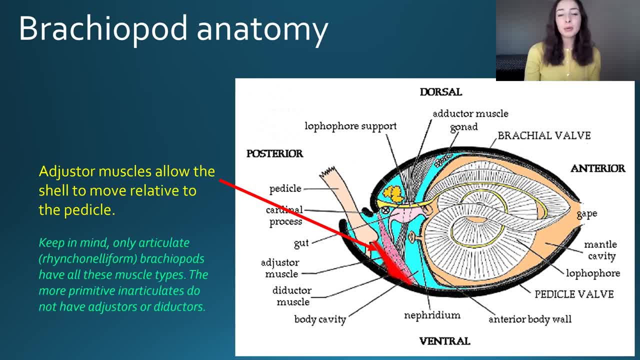 which allow the shell to move relative to the pedicle. And it's important to keep in mind that not all brachiopod types have all three types of these muscles: adductors, diaductors and adjuster muscles. Instead, some of them have just adductors and diaductors or, for example: 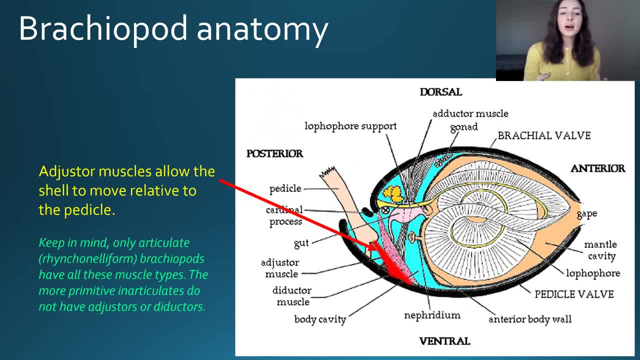 inarticulates only have adductors, kind of like bivalves, and they don't have adjusters or diaductors. And this is thought to be because inarticulate brachiopods are pretty primitively forms of brachiopods, whereas some of the articulate groups are a lot more well-evolved. 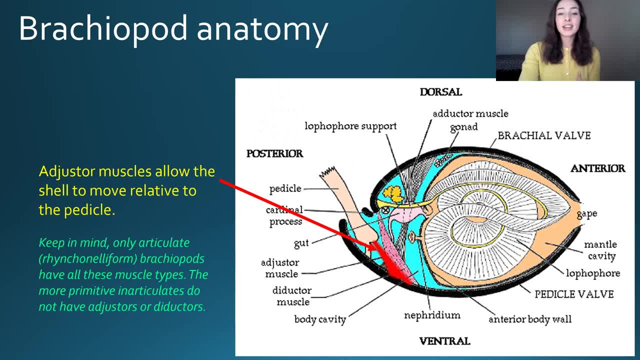 and so they have more muscle groups. But in general, as we label all of these characteristics on this one brachiopod diagram, we have to keep in mind that they're all kind of different, and we'll get into that later. when we talk about the classification of all the different orders. 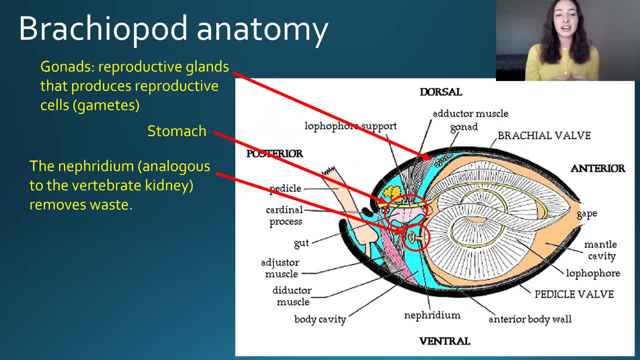 of articulates and inarticulates. So the last three things on this diagram that we haven't labeled yet are the gonads or reproductive glands that produce reproductive cells or gametes. And then we have the stomach here circled. and then we have the stomach here circled, and then we have 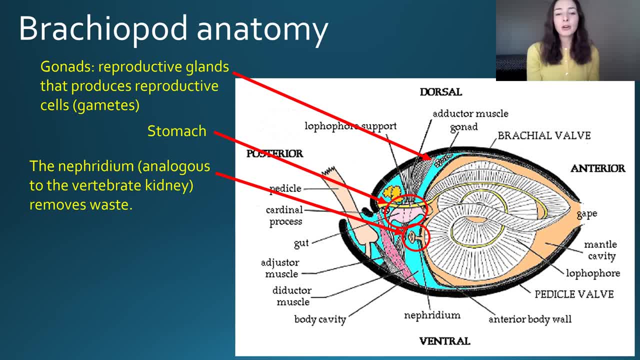 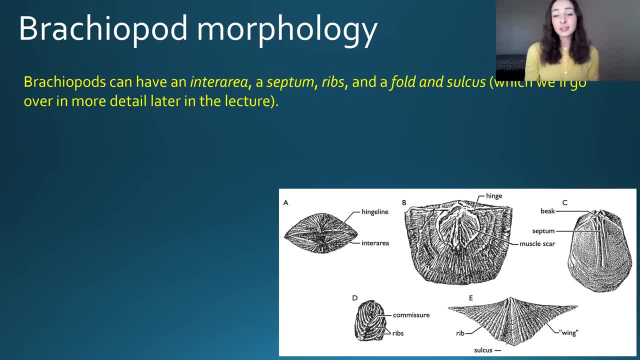 in pink. and then we have the nephritium, also circled here in the posterior part of the mantle cavity, which is what removes waste. So, getting into the morphology of the more fossil brachiopods and what you would need to identify brachiopods as fossils, brachiopods have what's called an. 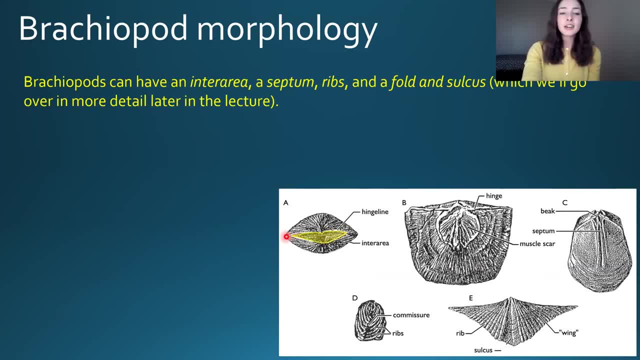 inter-area, So I just circled it here in yellow, And this area, as you'll see later as we get into the different classifications, will be important for diagnostic features later on. Additionally, brachiopods can have a septum, which is what we call a septum, and then we have a septum. 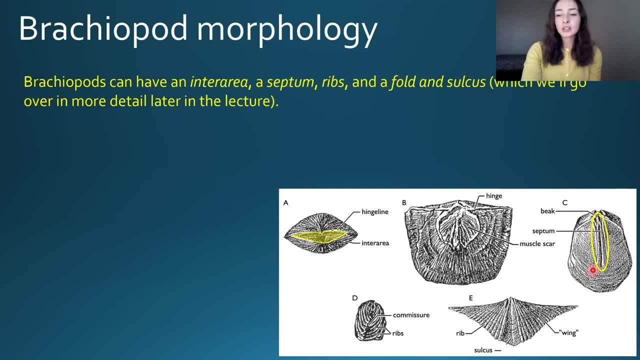 such as the group pentamerids which we'll talk about later. This picture is an example of those guys and they have a long septum in the middle of their valve here, And then they can also have ribs. A lot of the groups we'll talk about later have ribs where they have these ridges radiating. 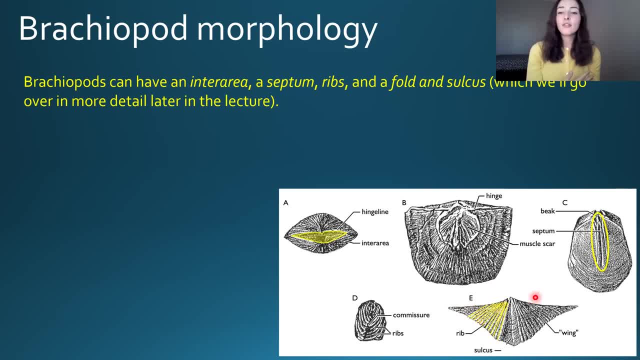 out from their hingeline. And then brachiopods can also have something called a fold and sulcus, and we'll get into this later, because there's not really a picture on this slide where you can see that at a good angle. So I'll show you some examples of a fold and sulcus later And then 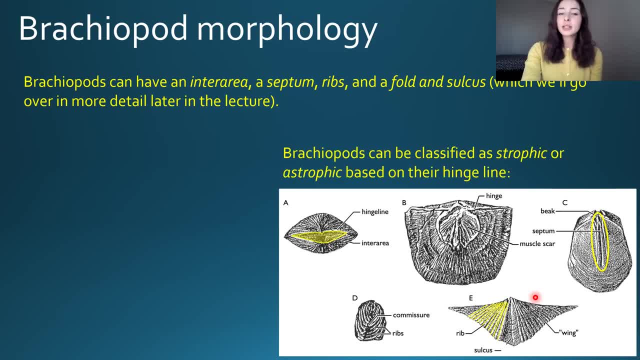 another thing important on this figure is the hingeline, which can either be classified as strophic or astrophic, And strophic just means pretty long and straight, as shown in figure B on this picture, And then astrophic means it's not really long and straight at all. 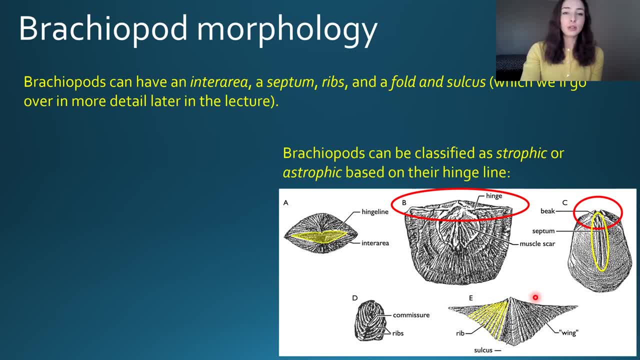 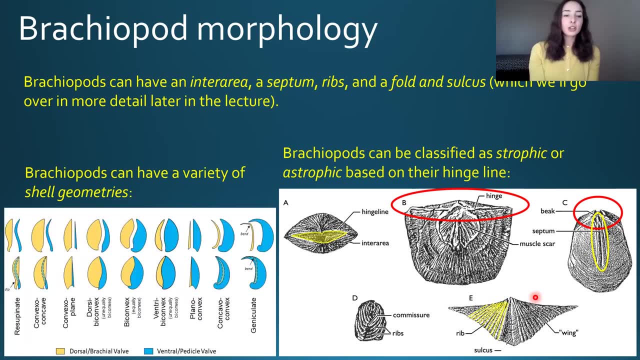 it's kind of curved and short, And that's another important diagnostic feature we'll show later during the classification slides. Lastly, brachiopods can have a variety of shell geometries and these are shown here. Like we mentioned earlier, there can be a larger valve and a 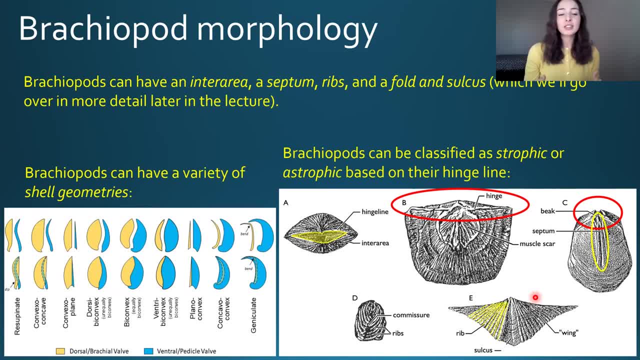 smaller valve, and then there can be a smaller valve, and then there can be a larger valve, and this can happen in a variety of ways. Brachiopods are incredibly diverse, as we mentioned earlier. So, as we see on the bottom left of this slide, 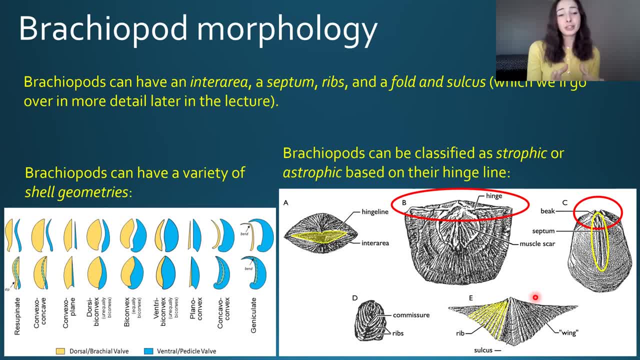 we see some different ways brachiopods can have their shells be shaped. So, for example, a typical shell morphology- we'll see later on when we talk about the different groups- is a biconvex morphology, where both valves are convex in their shape, And this can either be occurring. 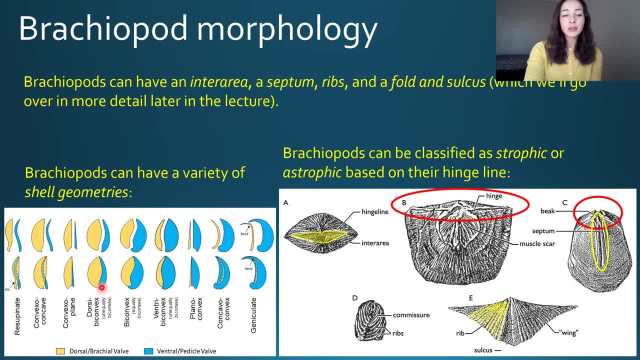 in a strongly convex way or a more gentle way, where they're both convex, but you know, they're not that curved. And then we also have morphologies where one valve can be planar or straight and then the other valve is convex, Or we can have one valve convex and one valve concave. 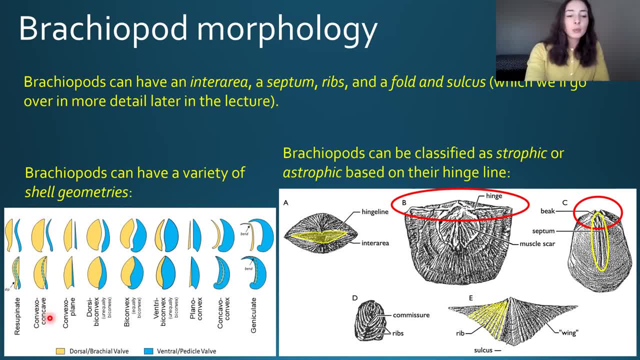 and this can either be called convexo-concave, depending on which valve is which, or concavo-convex. And then there are some more extravagant shell morphologies on the outside of this figure, but we won't be talking about those today. We're mainly going to be talking about biconvex strong. 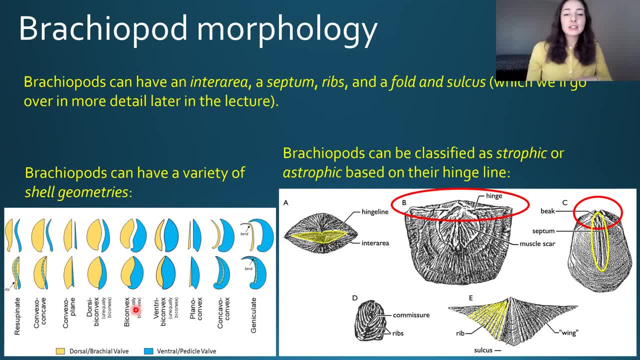 biconvex, concavo-convex and plano-convex. So keep in mind those kinds of terms and I'll show you pictures along the way as well, so you can keep that organized in your brain, But you don't. 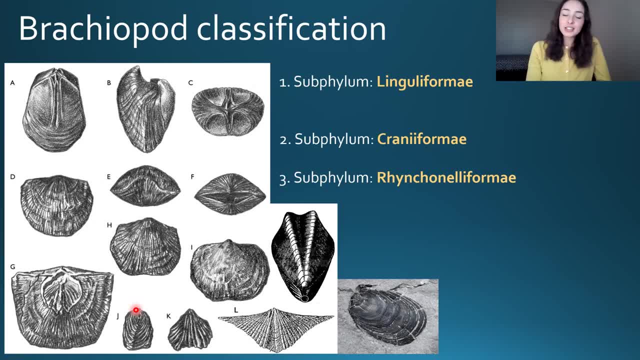 need to know every single one of these words. So, getting into the classification, we have three sub-phylums of the phylum brachiopoda. These include the lingula formae, the craniformae and the rinconella formae. I'm pretty sure I'm saying that right, but you know, we're just gonna. 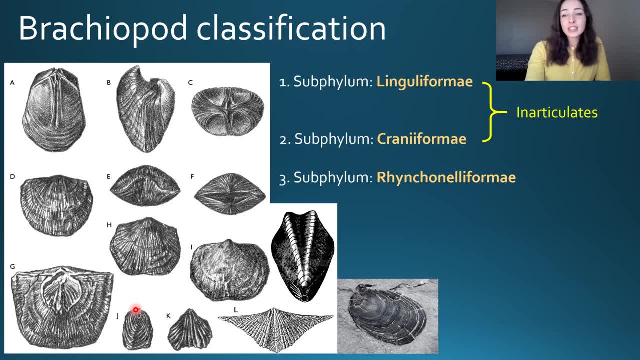 talk about it. Okay, so you heard me talking earlier about something called inarticulate versus articulate. This is because the old classification for these groups were lingula formae and craniforms being combined into inarticulates, which used to be a class but is now just kind of an informal. 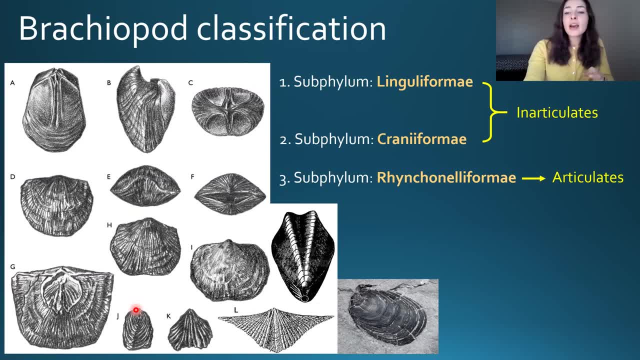 name or grouping of these two sub-phyla, And then the rinconella formae were called articulates rather than rinconella formae, And so the main difference: that people separated these two groups, because articulates form their shells with calcium carbonate And this is the typical calcareous. 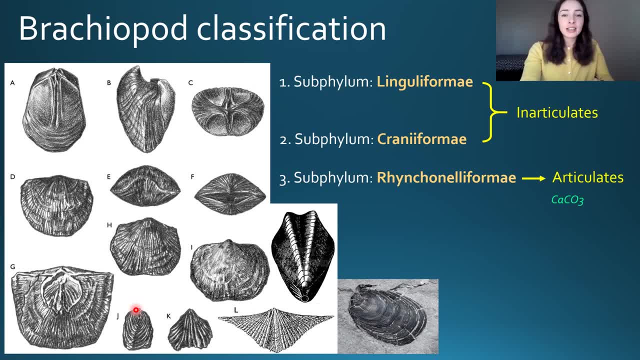 skeleton or shell type that pretty much all skeletonized invertebrates use. However, inarticulates used, and still use, calcium phosphate plus chitin, which is an organic material to make their shells, And so this was a very different and unique feature among the inarticulates, and still 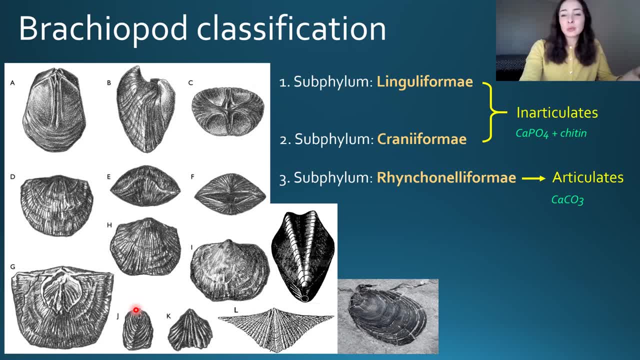 is today because there's still groups of inarticulates that live today, And this is why the inarticulates are so important. So now we're going to get into the more specific groups within the sub-phyla, in which we're going to talk about their specific features. So first we're going to 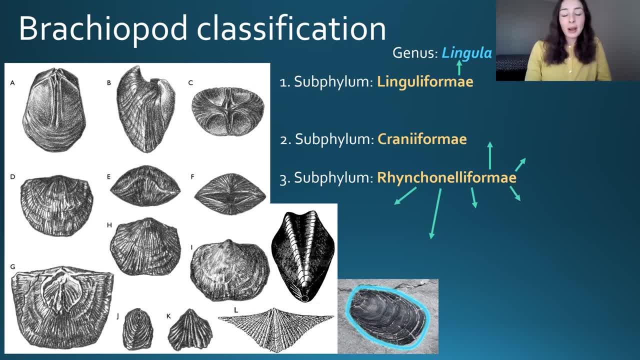 talk about lingula, which is the genus of the sub-phylam lingula formae, And then, unfortunately, we really don't have much to say about craniforms, so we're not really going to talk about those. But when it comes to the articulates or rinconella forms, we're going to talk about six orders of 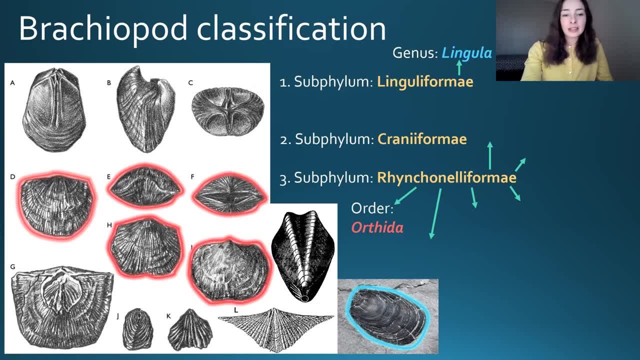 this sub-phylam, And these include orthids which are outlined in red in the figure to the left, strophaminids, pentamerids, spiriferids, rinconellids and terebratulids. So to get. 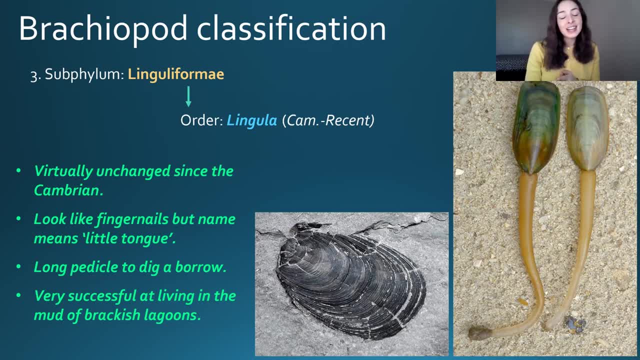 started with the genus lingula, which I just now realized that that label order is wrong. it should say genus, So lingula, the genus of the sub-phylam lingula formae, went from the cambrian to now And this genus has virtually gone unchanged since the cambrian. These are: 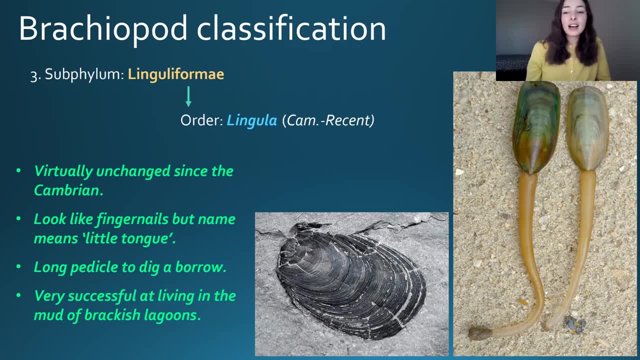 the two pictures we showed you earlier at the beginning of the lecture And, as you can see, life picture, which is a recent image on the very right, is really similar in appearance to the fossil in the bottom middle picture, And this is because they just haven't changed much In terms. 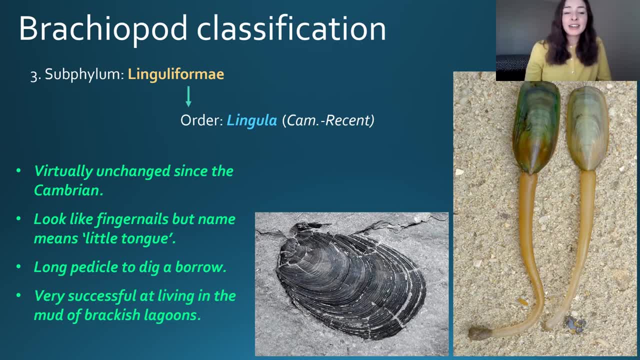 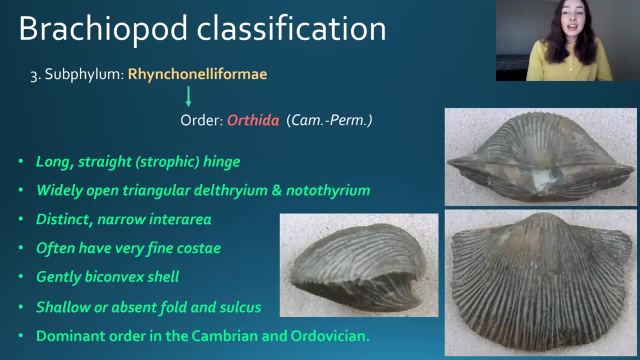 of what they look like. I kind of think they look like fingernails, but their name means little tongue, So you can also think of them as a little tongue, I guess. And then they have a long pedicle to dig and burrow And they are very successful at living in mud in brackish lagoons. 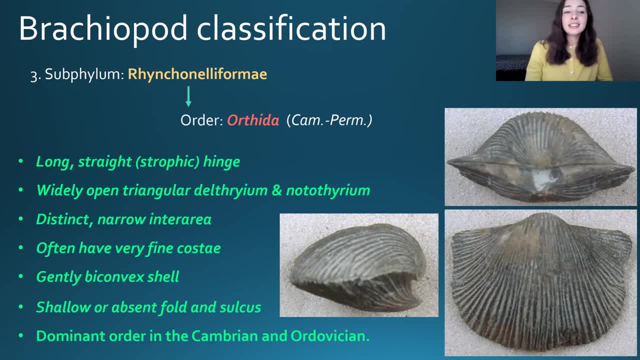 So let's start with the articulates or the rinconela forms, And in this sub-phylam, we're starting with the order orthoda. This is an order, so keep in mind that the rest, from here on out, are orders, not genera. And this order of orthids went from the cambrian to the permian. 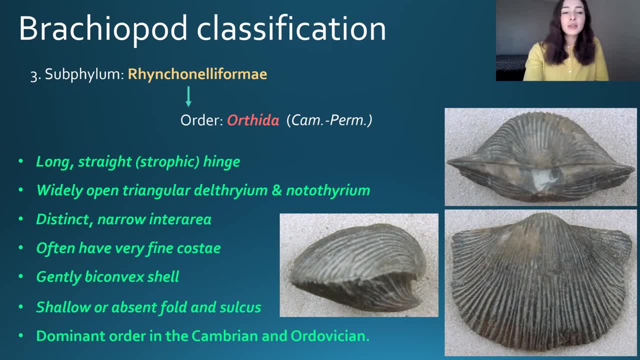 And some diagnostic features that you can use to identify orthid fossils include its long, straight strophic hinged line shown here on the right. Also, it has a wide open triangular deltherium and nodotherium, which are just fancy things that are not related to the genus lingula. 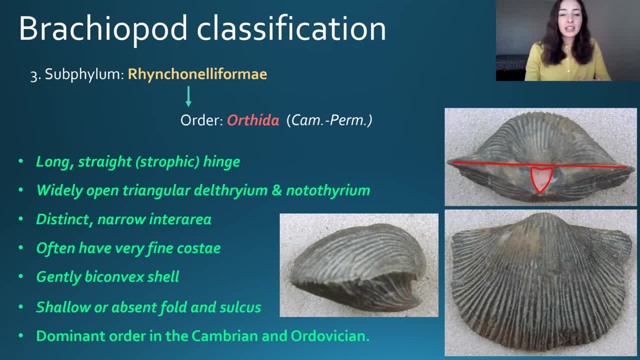 Nototherium, which are just fancy terms for part of the pedicle opening. They're kind of plates that cover it and can be either closed or open, And so we can see that their shape in this case is triangular and open, And then they have a distinct narrow inter area, as we can see. 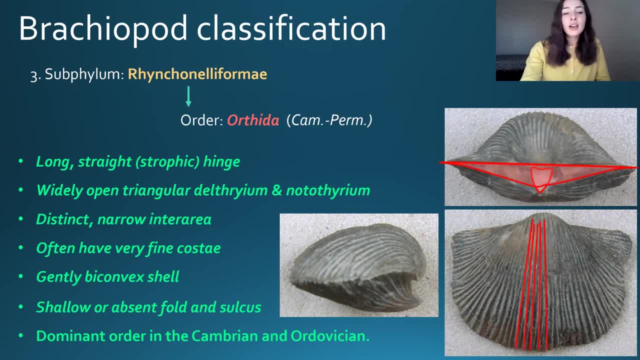 highlighted on the right again. And then they also have very fine costae, which is a fancy word for lines radiating from the hinge, that when they're not raised or ridges they're called costae or whatever you want to use, And when they are raised or ridges they're called ribs or ribbed. 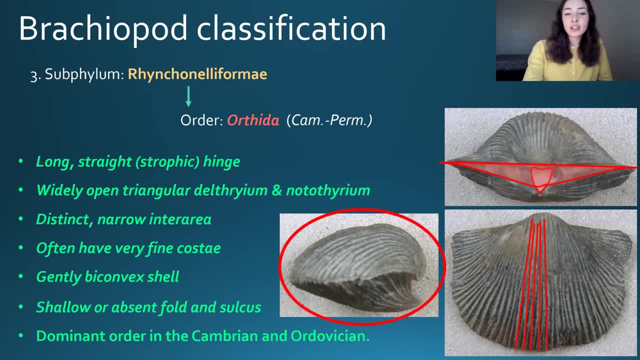 costae. And then they are gently bi-convex in their shell shape and they often have a very shallow fold and sulcus or no fold and sulcus at all. Again, I haven't shown you a great picture of a fold and sulcus yet, but I promise when we get to spiriferids you're going to see a. 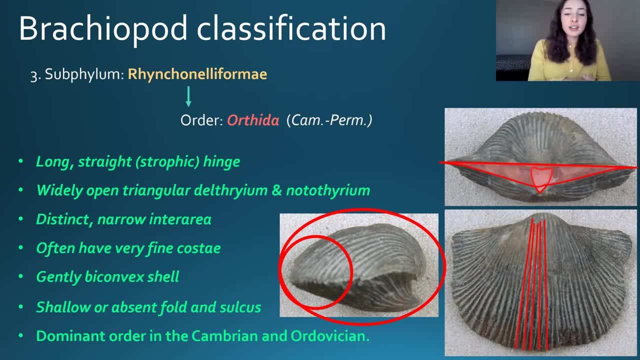 great image of a fold and sulcus. It's basically when at the front of their shell they have a big fold or dip in it and it's just called a fold and sulcus. So we'll see that later. In terms of the evolutionary trends of orthids throughout Earth's history, they dominated in. 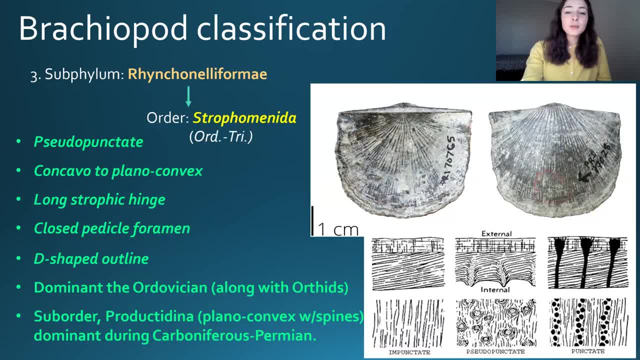 the Cambrian and Ordovician, so early Paleozoic. Next we have the Strophominids. Strophominids have a very distinctive feature of being pseudopunctate, unlike any other of the brachiopod orders, And I haven't yet explained what this means. So if we look at the picture, 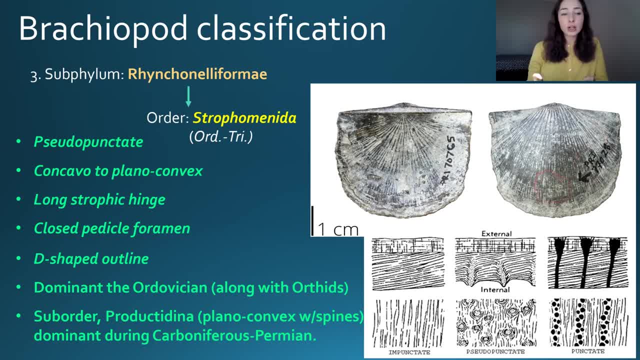 to the bottom right we have this figure showing the internal structure of brachiopod shells. So the top row of that figure is showing the brachiopod shells in cross-section, whereas the bottom of the figure is showing them looking at them head on And, as we see, some brachiopod types have shells with pores or 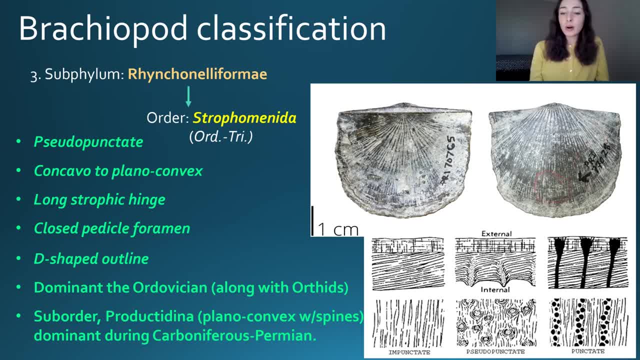 punctures, and these are called punctate, as we can see in the far right, Whereas some brachiopods don't have any pores or punctures, and these are called impunctate, as we see on the very left of the figure. And then, lastly, in the middle, we see some punctures or holes that 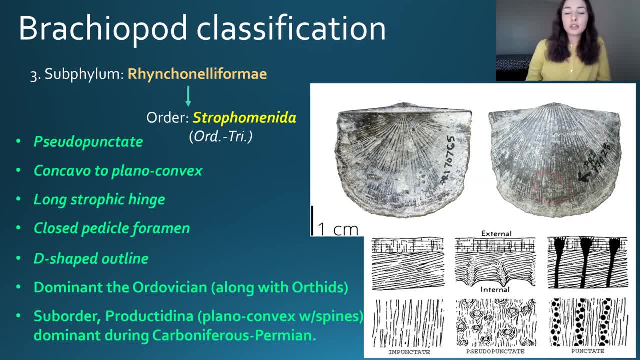 kind of go halfway through the shell but not all the way through, and these are called pseudopunctate, So they appear like they might have pores but they don't, And this is a diagnostic feature of strophominids. Additionally, strophominids are typically concave or convex. 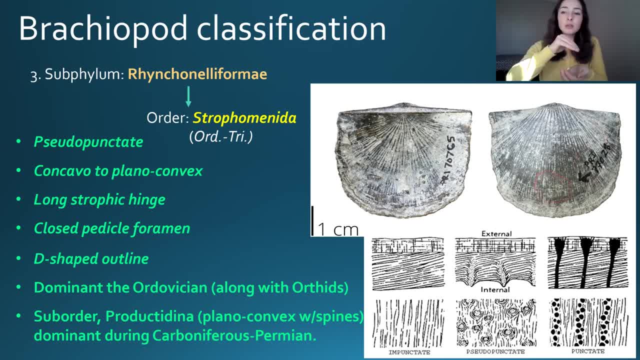 to plano-convex. So they have one shell that's convex with another shell that's concave, or they have one shell that's convex with their other shell as planar or straight, And they have a very distinctive and long strophic hinge line, similar to the orthids, but typically they have 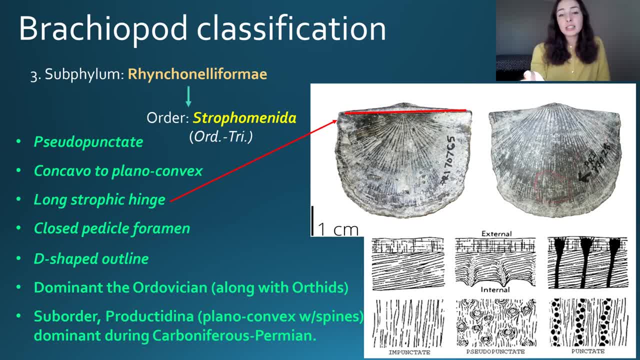 an enclosed pedicle foramen or pedicle opening, And so that distinguishes them from the orthids in that they don't have that larger interior area and they don't have that open pedicle opening. Additionally, they tend to have this really diagnostic d-shaped outline, as we can. 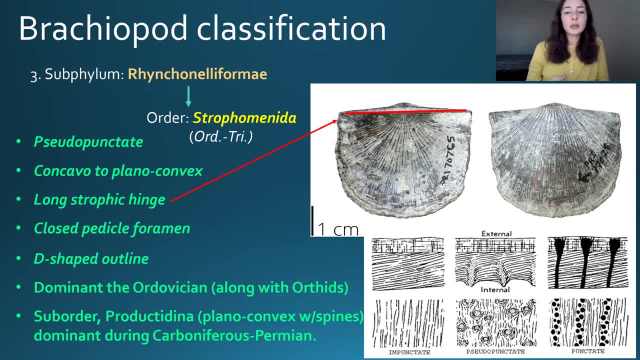 see in the image, and they were dominant during the ordovician, along with the orthids. However, this is not where we'll leave the strophominids. They had another group, which was a sub-order, called the productids. These were plano-convex with spines, which makes them pretty easy to 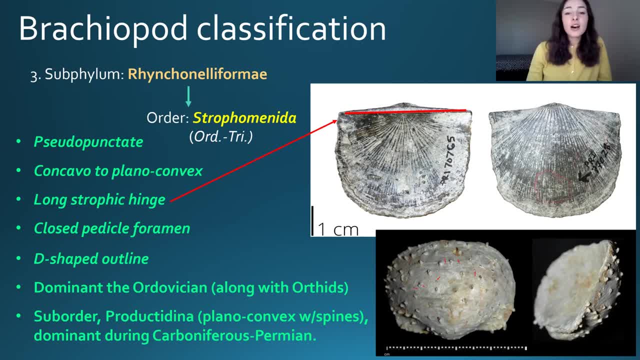 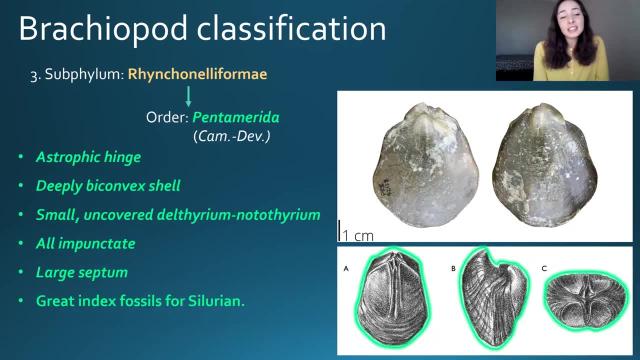 recognize. However, spines are always preserved, so you kind of have to use other features as well. But these productids were dominant during the carboniferous to the permian, so late paleozoic. Next order of the rinconella forms that we have is pentamerids. 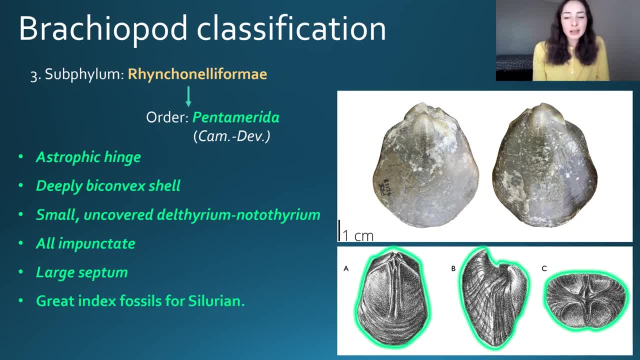 The pentamerids went from the cambrian to the devonian, so pretty short time scale, making them pretty good index fossils. And these pentamerids typically had an astrophic hinge line, so curved, small, not really long and straight like the strophic ones we saw in the orthids. 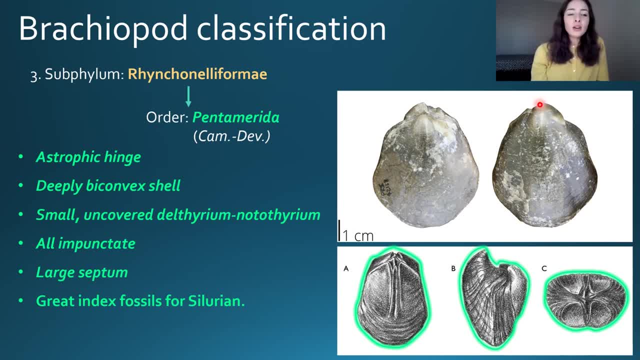 and strophominids- And this is one of their really diagnostic features- along with a deep biconvex shell shown in B in the figure at the bottom, And they also had small uncovered deltherium and nototheriums and they were all impunctate. So if we remember from the 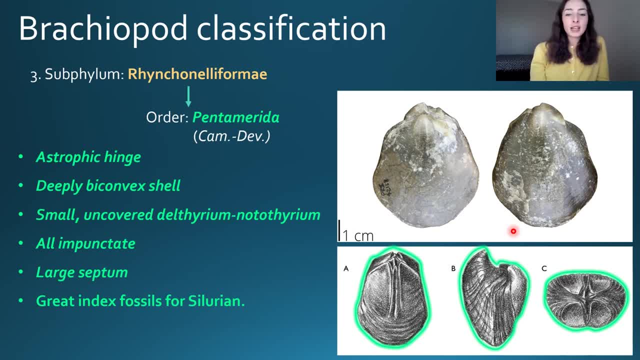 previous slide we talked about the strophominids typically being pseudopunctate, which was really diagnostic of them. However, in the pentamerids they were all impunctate, so they had no pores or holes or whatever in their shells And they had what's called a septum, which we talked about on. 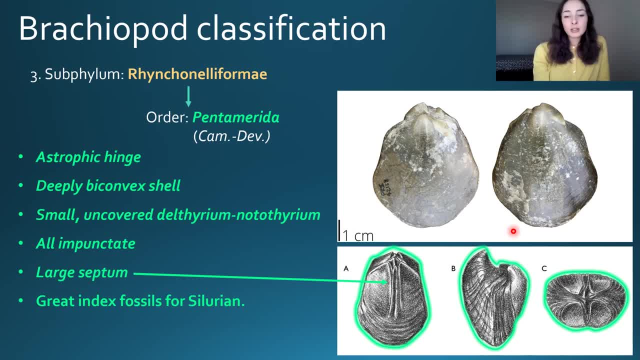 the morphology slide, And this is really diagnostic for pentamerids, because they're a very long and distinctive septum going down their bowels And lastly, they make great index fossils for the Silurian period, which was early-mid-Pileozoic. Then we have the spiriferids. 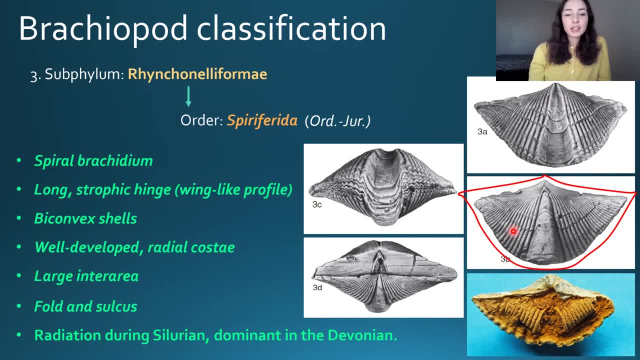 The spiriferids went from the Ordovician to the Jurassic. If you have a really well-preserved spiriferid brachiopod, you might be able to break it open and find the brachydium or the local force support that we talked about earlier, preserved in the brachydium. 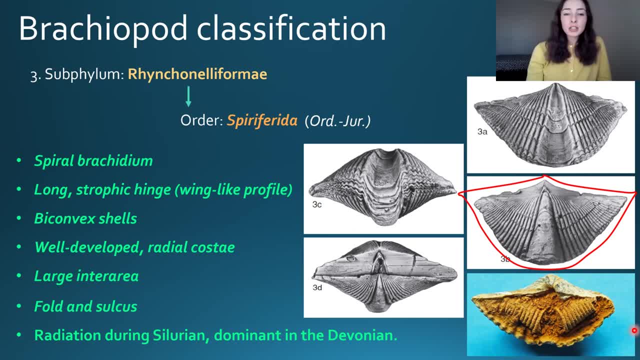 So this is a very well-preserved brachiopod. Remember that we talked about that. the local force support, or brachydium, is calcareous, which is why sometimes it gets preserved. This makes it a great diagnostic feature when preserved, because the brachydium can take different morphologies depending on the 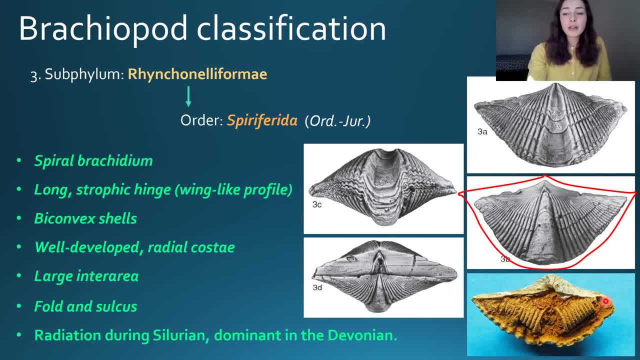 order or class of brachiopod you're looking at. For example, in the spiriferids it had a spiral brachydium, as we can see here at the bottom, And this was really diagnostic of that order. However, 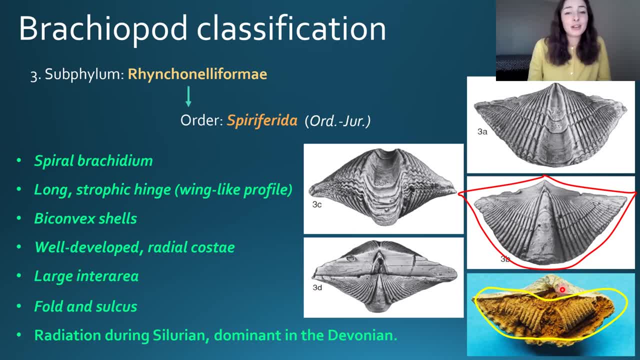 they have a bunch of other diagnostic features that you may not need- the brachydium of spiriferid- because they're so distinguishable on their own, As we see. they have a long strophic hinge line and a wing-like profile, as we see on figure 3b to the right here. They also had pretty bi-convex. 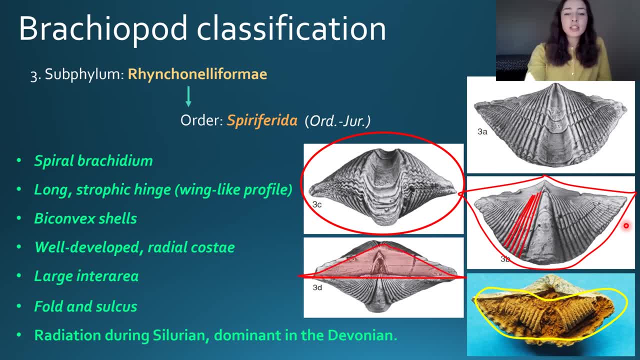 shells and they had well-developed radial caustic. Additionally, they had a large inter-area and often had a really distinctive fold in sulcus. This is finally the good picture I was hoping to show you guys of the fold in sulcus. You can see here that there's a fold in both of these shells. 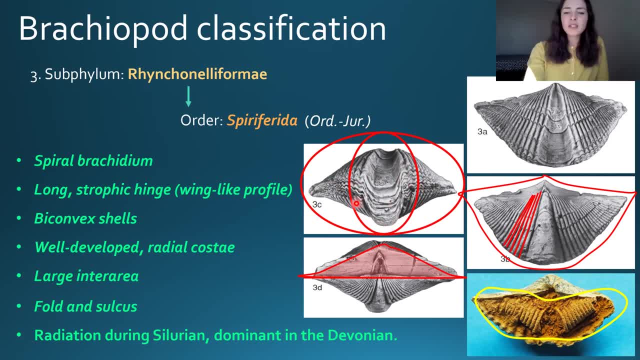 making the commissure, which is where both the valves meet up, kind of deformed in that area. But the commissure follows that fold and so that fold and sulcus, where the fold is the more humpy kind of anticline part if you're a geologist, and the sulcus is the u-shaped part that we see on the 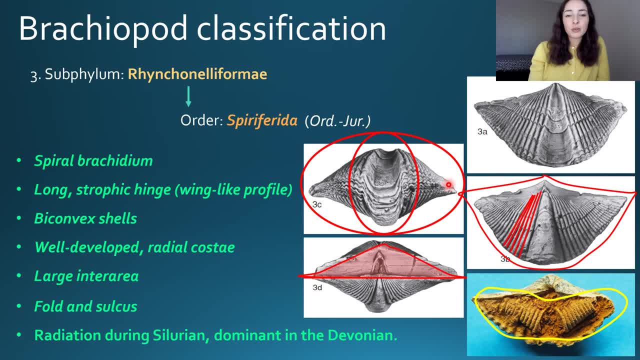 top valve here in this picture. that is a really distinguishing feature for some of the groups of spiriferids. And lastly, for the spiriferids, they went through a radiation or major diversification during the Silurian period and this is a really interesting feature for some of the groups of. spiriferids. And lastly, for the spiriferids, they went through a radiation or major diversification period- and this is a really interesting feature for some of the groups of spiriferids. And lastly, for the spiriferids, they went through a radiation or major diversification during the Silurian period. 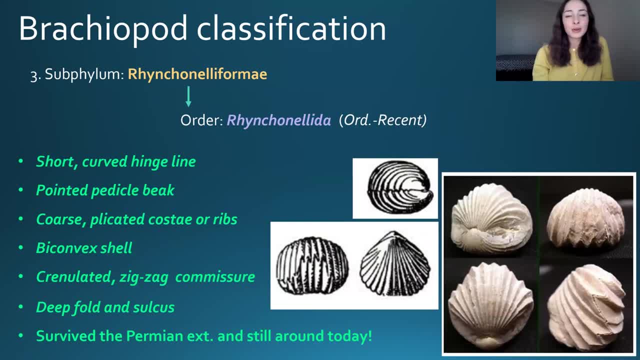 and then dominated during the Devonian. The second to last order for the Rinconella forms that we have is the Rinconellids themselves, and this order went from the Ordovician to now. Rinconellids had short, curved hinge lines, so they were astrophic and they had a pointed 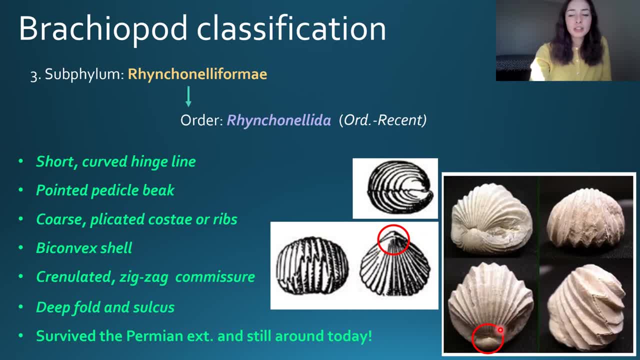 pedicle beak. As we can see in the bottom right picture, we have this circled area with this beak here, which was pretty pointy. Additionally, they had coarse costae or ribs. as we can see, they are steep ridges. And then they also had a pretty strongly biconvex shell and they had 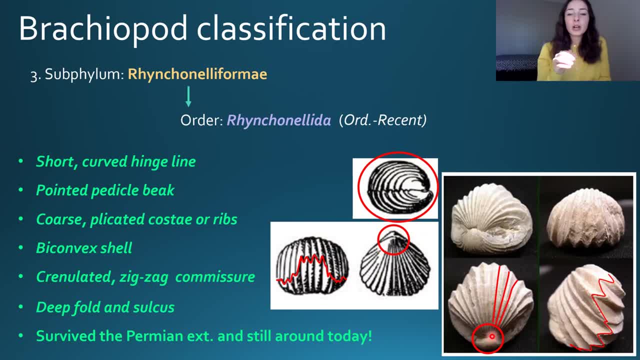 a craniolated zigzag commissure. So the commissure where the shells meet was very zigzag, as we can see in these figures, And we can also tell in the figure looking straight on the commissure to the left. we have a very deep golden sulcus present in this order as well. 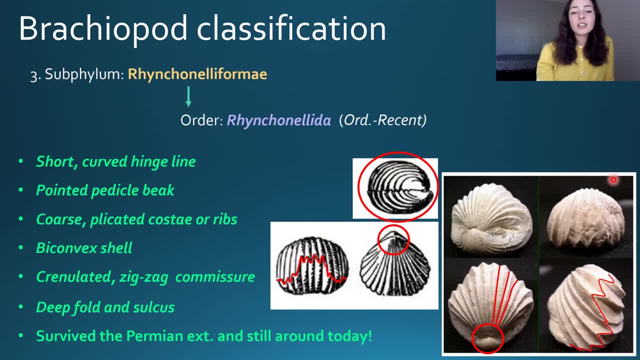 The Rinconellids survived the Permian extinction and are still around today, in the Rinconellid era, And they're one of only two orders of articulate brachiopods that survived until today. The other order that is still around today is the Pterobrachylids. The Pterobrachylids. 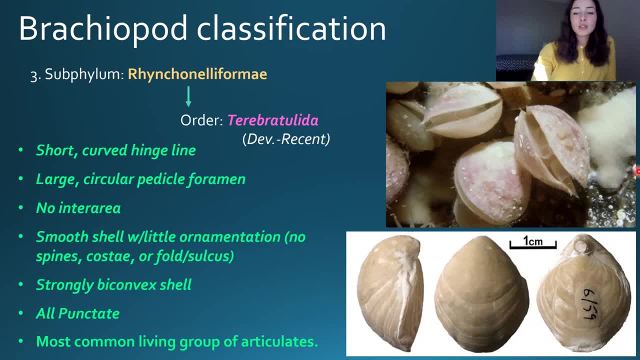 went from the Devonian to now and they are characterized by a short curved hinge line. so they are astrophic. They have a large circular pedicle foramen or opening, shown here in the bottom right, and they have no inter area and they have a smooth shell with little ornamentation. so no spines, no costae. 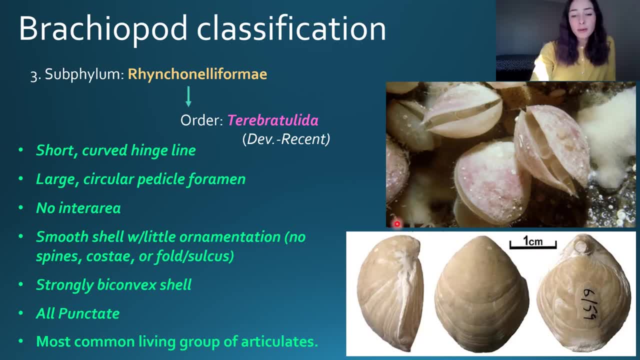 They have typically no fold in sulcus and they are typically strongly biconvex and they are all punctate. They all have pores or holes that go through their shells And we can see a picture of them in life at the top right, and they are the most common currently living group of articulate brachiopods. 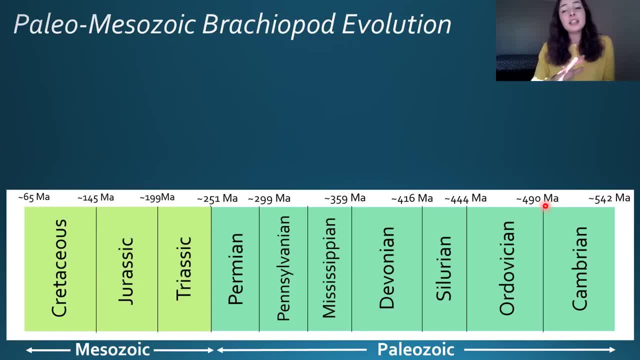 Lastly, we'll just recap the brachiopod evolution, because there's a lot of terminology, a lot of names, a lot of groups, a lot of orders, so we need to recap the evolution just to make sure we're all on the same page. 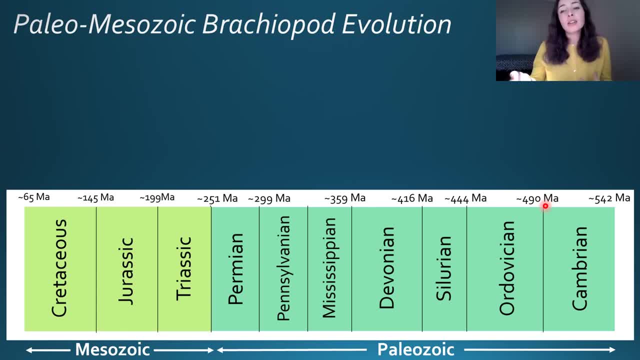 This is a timeline from the Paleozoic on the right to the Mesozoic on the left, And as we start in the Cambrian we had the lingula, foramen and crana formae sub phyla of the phylum brachiopoda. 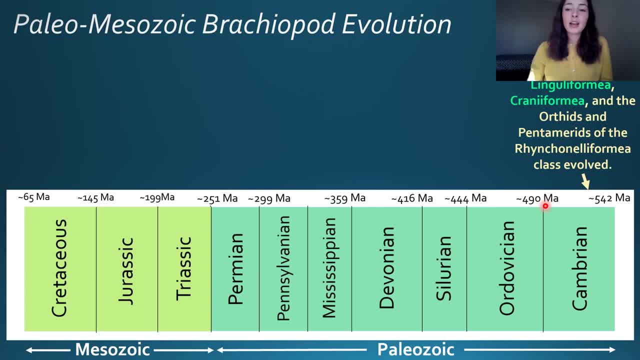 evolve in the Cambrian. And then we had the orders Orthoda and Pentamerida of the sub phylum rinconela foramen also evolve in the Cambrian. To make it a little bit easier to go through the evolution of these groups, we have the inarticulate Shonan-Green and we will have all of